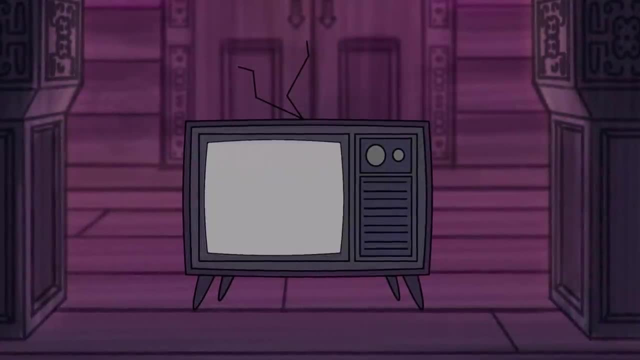 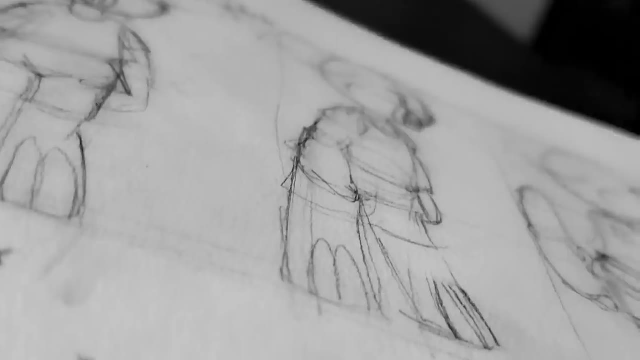 churning out episodes of that series, and I wish you well on all of your animated projects. I did notice, though, that a lot of comments on the first video were from disappointed people who said I didn't really teach them how to make an animated series. But I think what they meant. 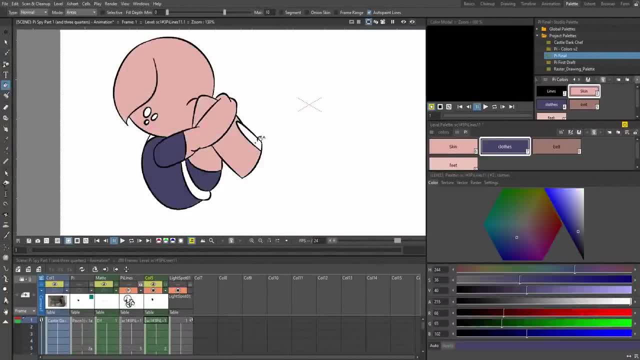 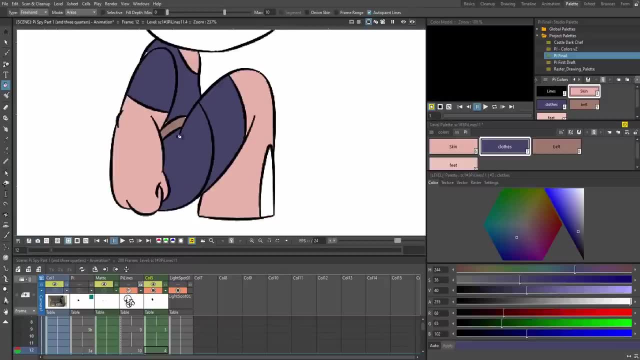 to say is that I didn't teach them how to make animation itself. Since that video was about making an animated series. going into it, I had already assumed that the viewers would know how to make animation, since making an entire series is a way bigger project. But as it turns out, 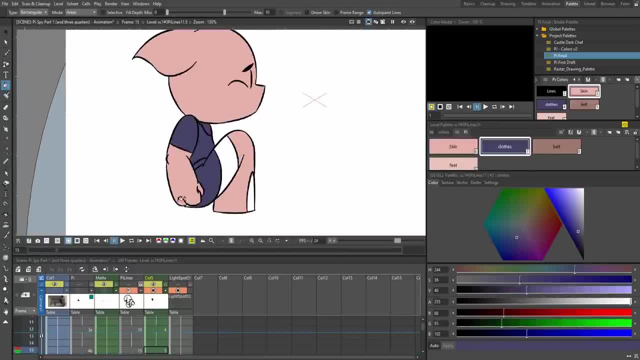 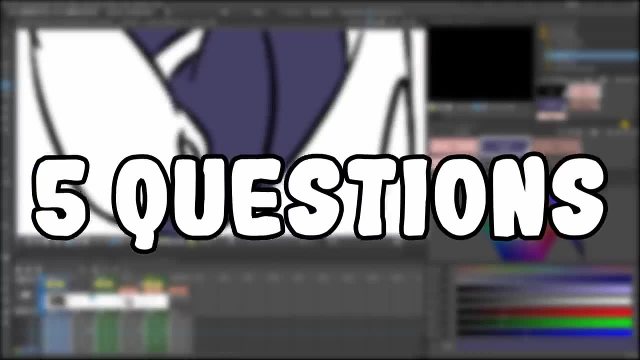 a lot of you out there want in on this animated series stuff, but you don't know how to make animations. So today I'm here to answer five very important questions so you can get started making your own 2D animation. Make sure to stay tuned until the end, because at the end of the video I have a huge announcement. 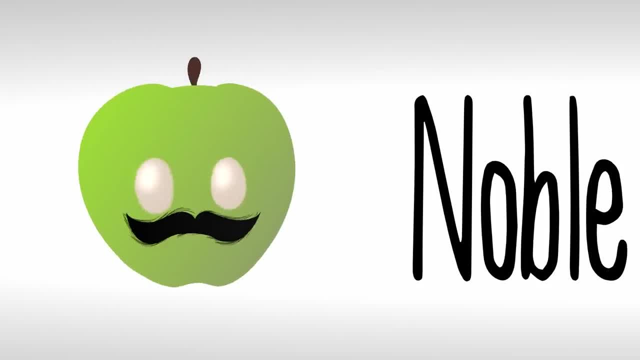 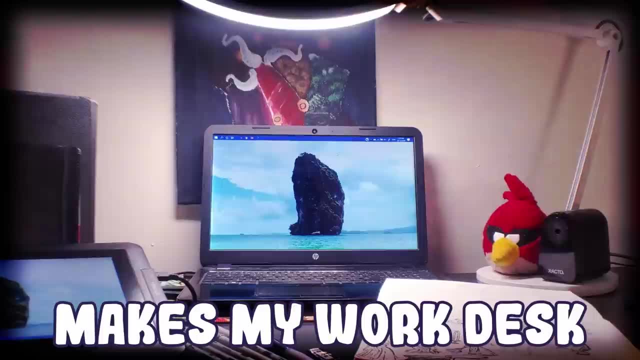 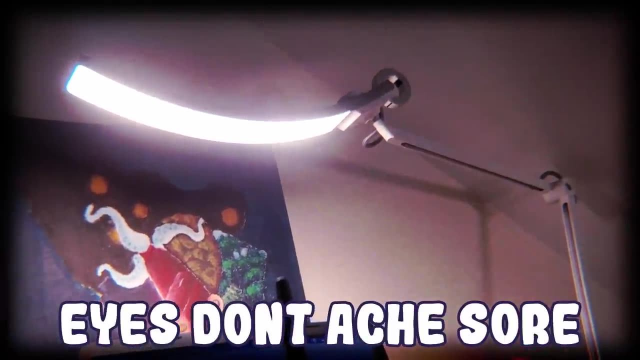 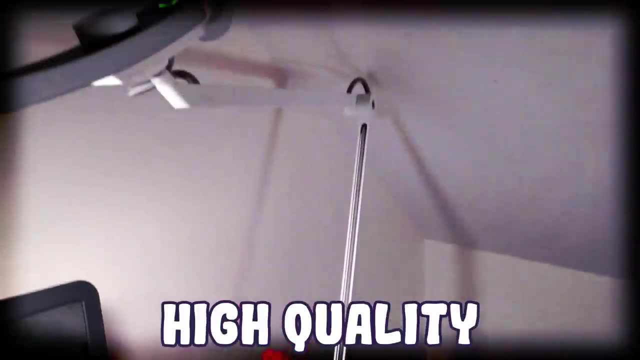 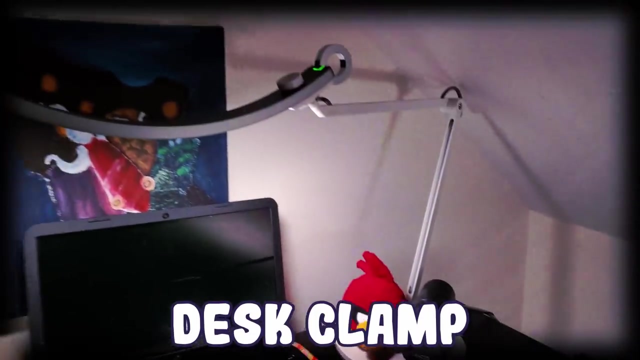 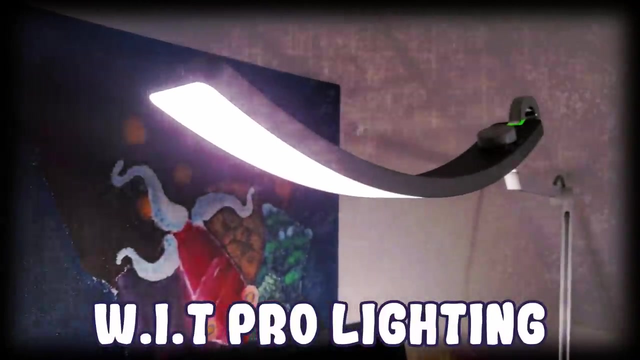 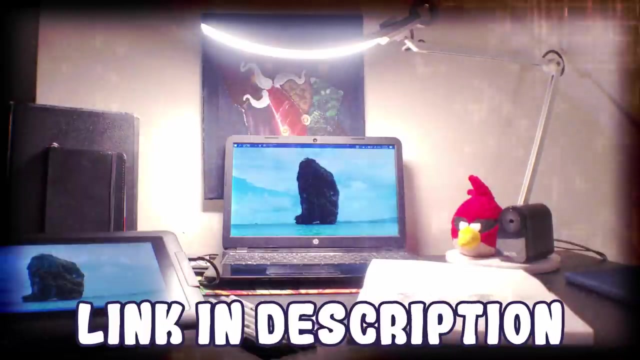 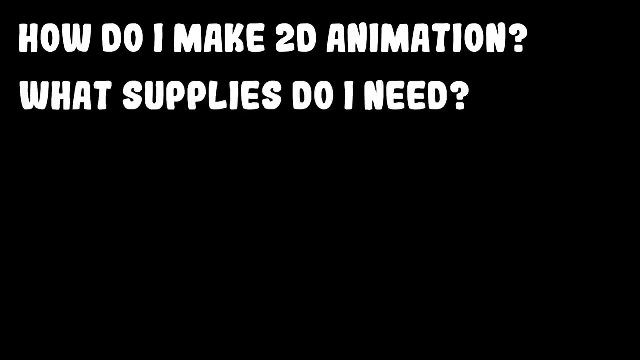 to make about this channel. Make sure to stay tuned until the end, because at the end of the video I have a huge announcement. The five questions are: How do I Make 2D Animation? What do I need to make 2D Animation? Should I Share My Animation? 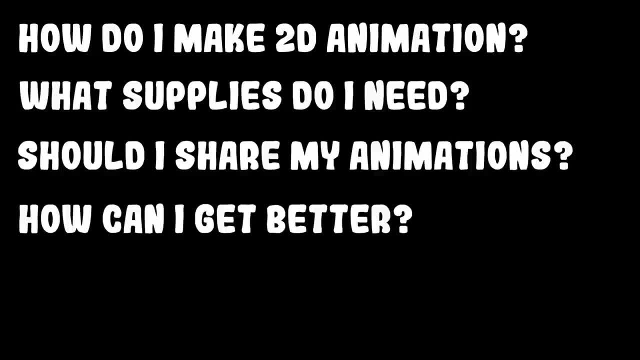 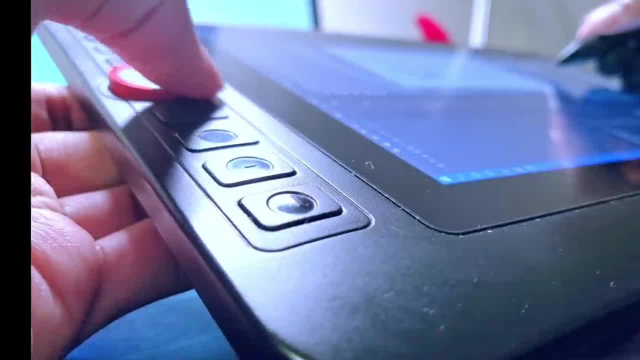 Animations, Where and how. Once I start, how do I get better? How long will it take to master 2D animation? So let's start with the first question: How do you make 2D animation? 2D animation is: 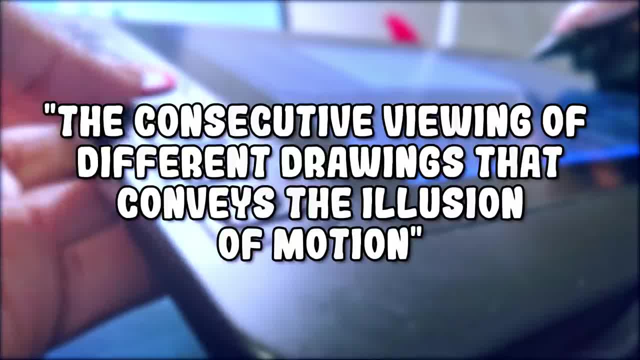 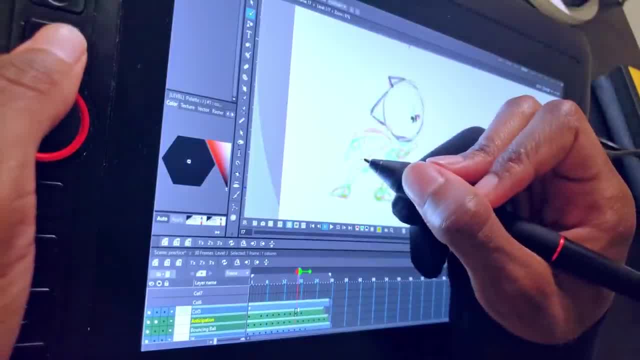 basically the consecutive viewing of different drawings that gives the illusion of movement. You can create this effect by using software to draw your individual frames and then export them to a video file for viewing them in succession. I recommend that you use the free 2D animation. 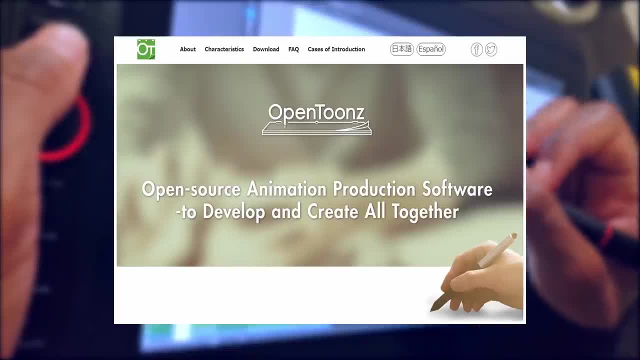 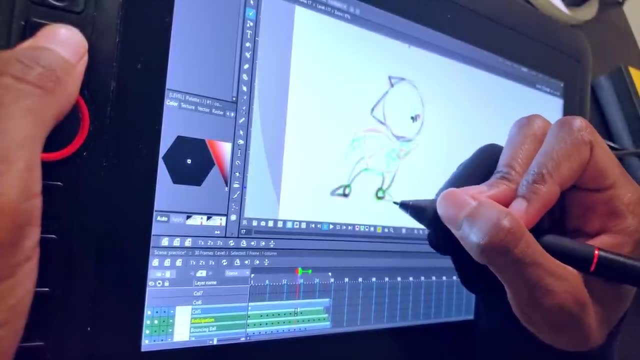 software, OpenToonz, to start making your animations. It's a little bit of work to get used to, but trust me, it's worth it in the long run. In addition to that, I recommend that you download a video editing software to compile all of your animated scenes. I use DaVinci Resolve. 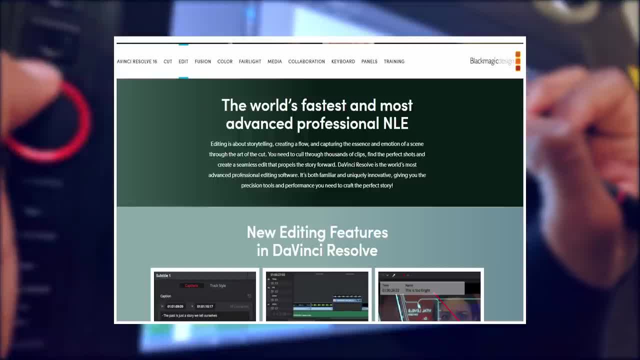 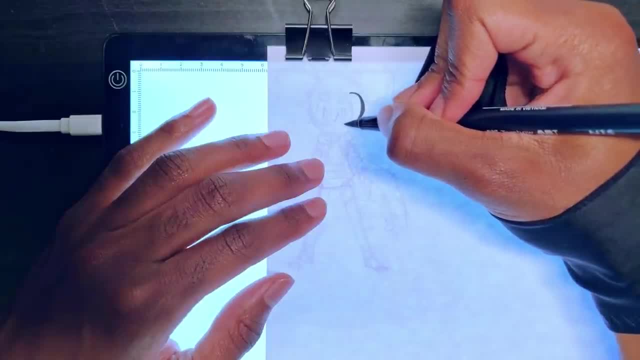 because it's capable of almost anything and it's free. You can also make animations traditionally by using special animation paper and a camera to capture your frames. But in order to keep this video as simple as possible, I'll stick to the faster and easier digital animation. 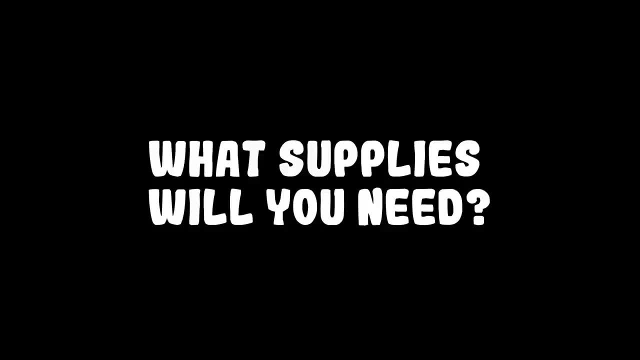 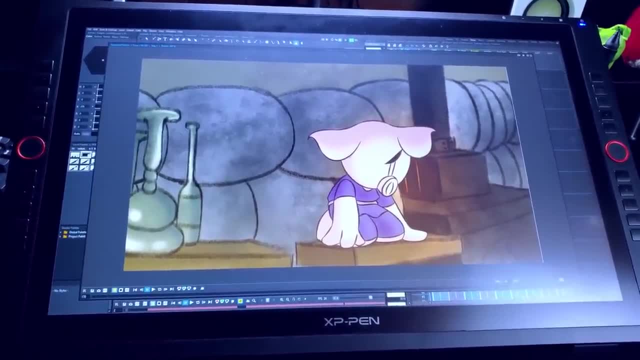 What do you need to make 2D animation? What you'll need to make animation is a capable computer, a drawing tablet and an animation software. If you plan to make large animated projects with lots of layers and effects, I recommend getting a computer with a decent 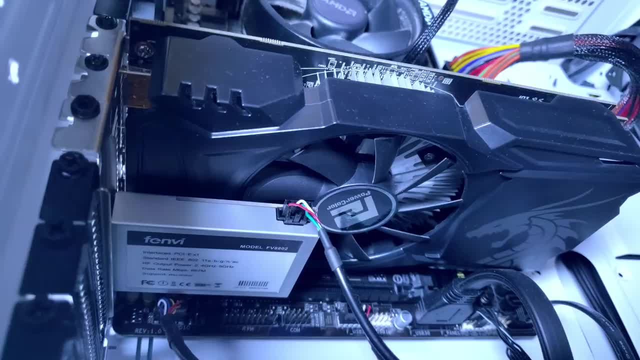 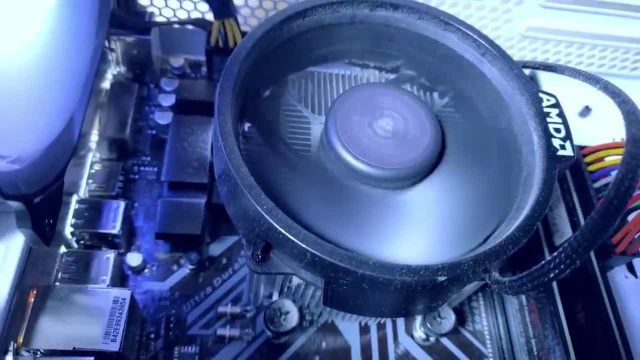 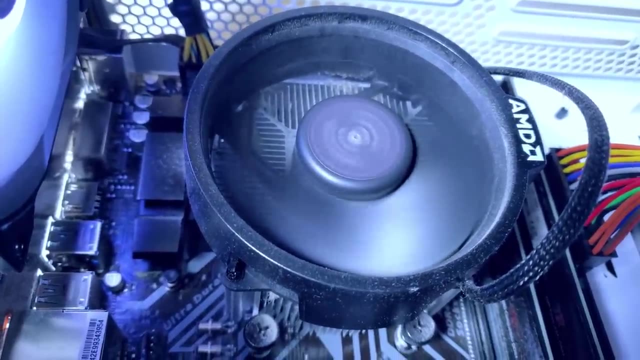 processor and graphics card. AMD Ryzen processors are great for creative work because they offer multiple threads for multitasking at an affordable price. This will cut down render times and speed up your complex workflow. If you're looking to just make simple animations, then your run-of-the-mill laptop will probably 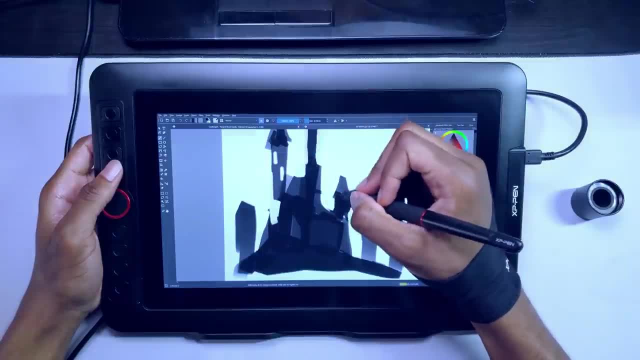 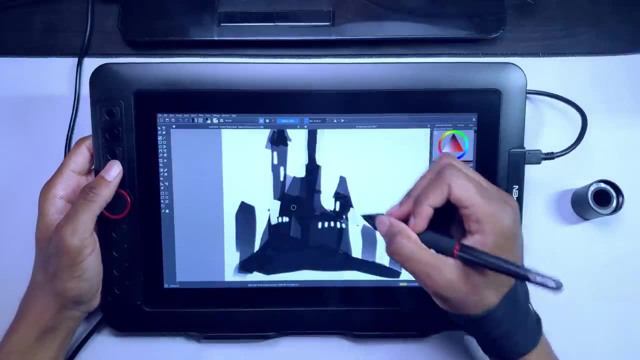 be fine for 2D animation at least. A drawing or graphics tablet is a device that you connect to your computer to make drawing easier and more natural. When you plug it in, it replaces your mouse with a pen, mimicking the traditional way of drawing with a pencil and paper. There are two kinds of drawing. 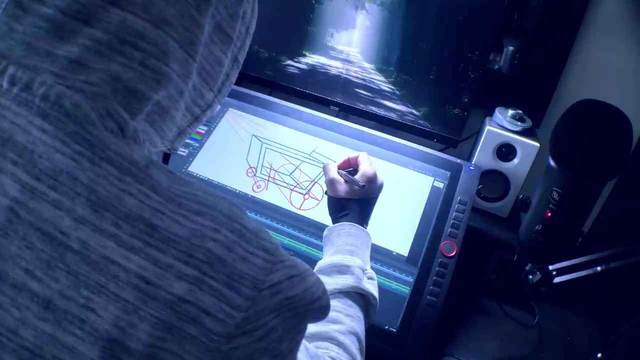 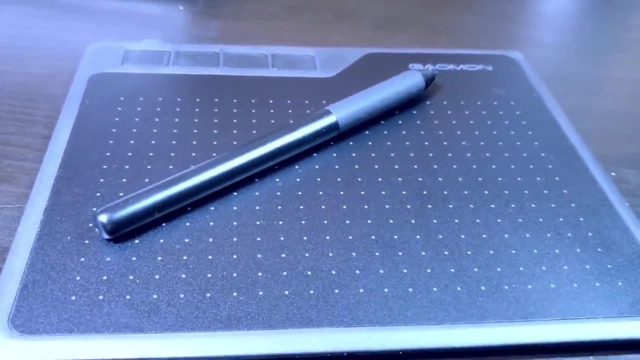 tablets, pen displays, which come with a display and act as an additional monitor, and pen tablets, which don't have a display but are mapped to your computer screen to coordinate the pen. Pen displays are easier and more natural to use, but they're much more expensive. 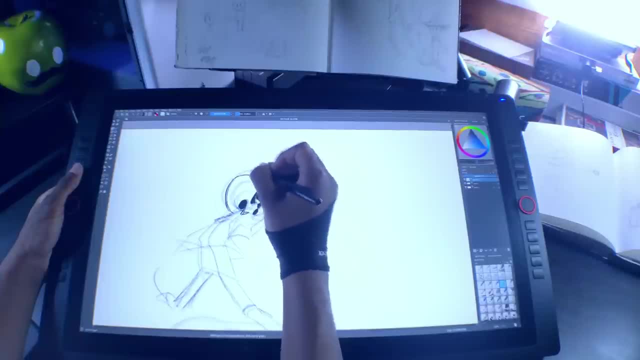 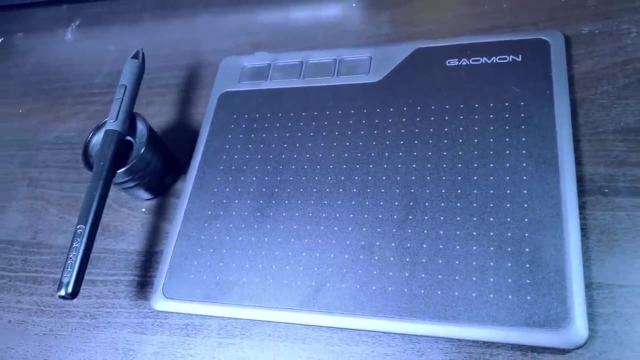 Pen tablets take some time to get used to, but are much more affordable. My advice is that, if you're on a budget, buy a pen tablet to help you get used to the world of digital art, After you've gotten used to the programs you're going to be using and you've established 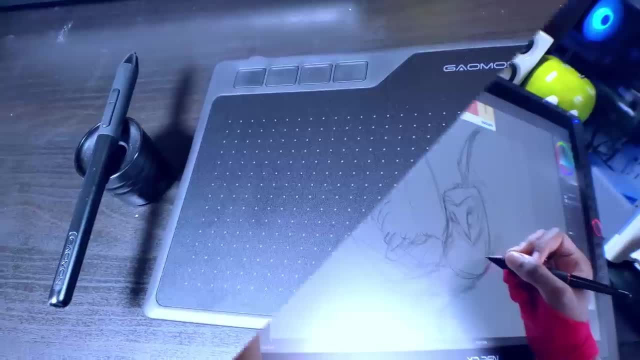 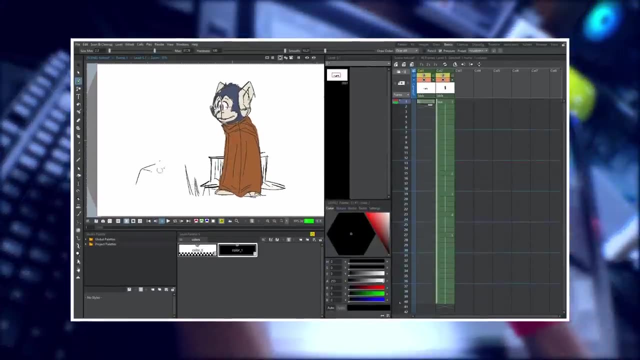 a basic workflow, then you should go for the more expensive pen display, But if you're not on a budget, then you can go with whatever your heart desires. By the way, here is an easy-to-follow animation tutorial for those of you who have purchased. 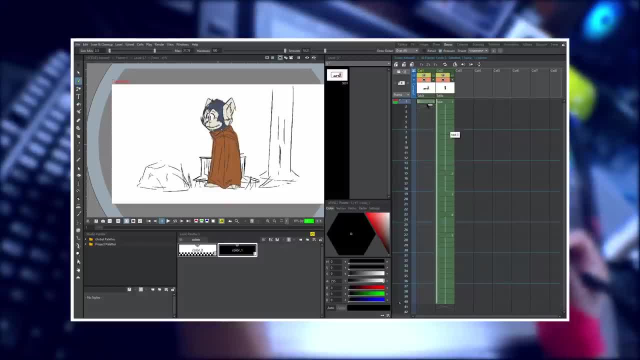 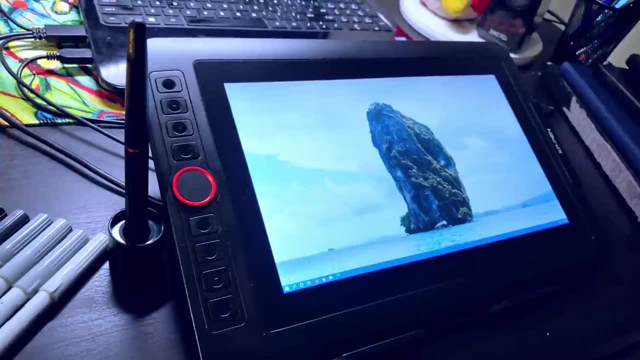 these materials and have downloaded OpenToonz already. If you're ready to go, I'm not going to stop you, Just click the link in the card. I also want to mention that you can buy anything you see here on my personal Amazon store. 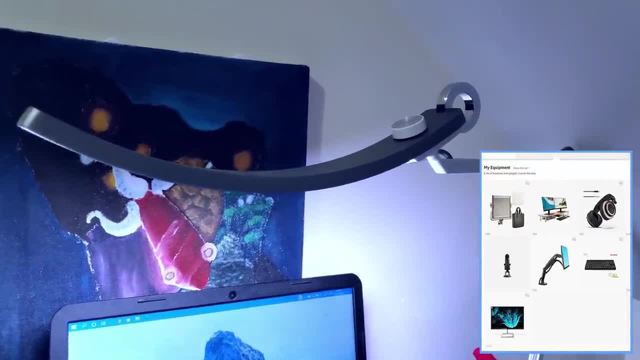 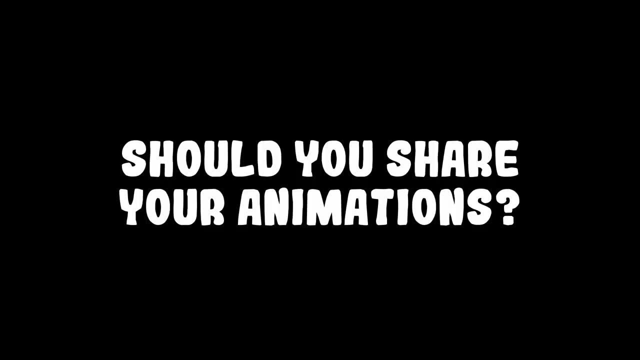 which is full of all the tried and trusted products that I've used over the years. Since Black Friday is coming up, I'd take a look and see what items you may consider buying on sale in a few months. Should you share your animations Where and how, It's completely up to you whether or 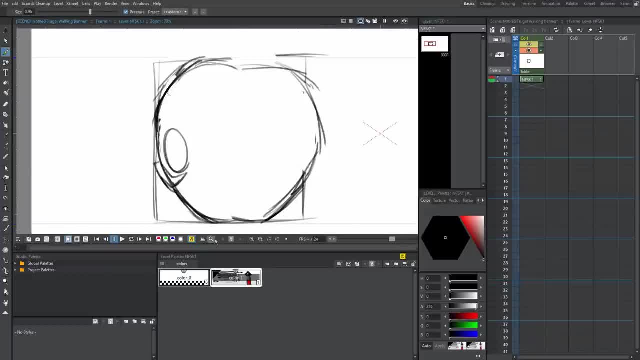 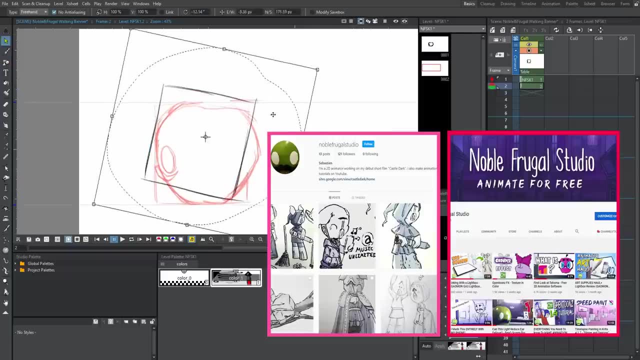 not. you want to share the animations you make with the world. An easy and affordable way to share them is on social media like YouTube, Instagram or any other online community. If you're interested in practicing animation and getting better, then I recommend that. 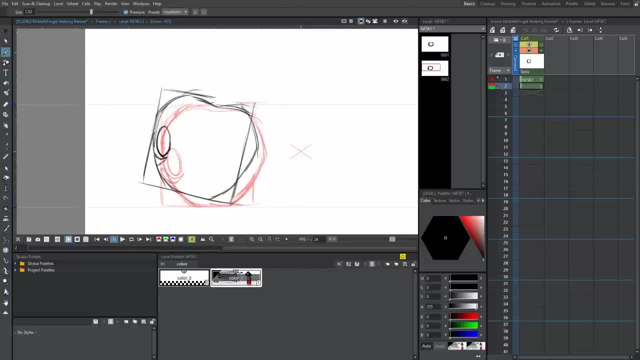 you join our Discord channel. We host challenges aimed at beginners and those looking to improve their skills in animation. Winners are actually featured on my channel, so if you join, give it your best. Anyway, if you're looking to make animated shorts or an animated series, then I recommend. 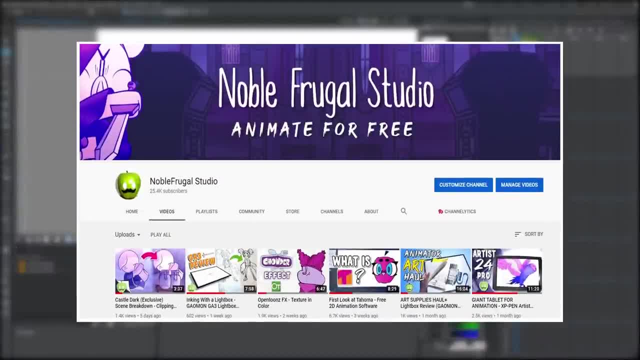 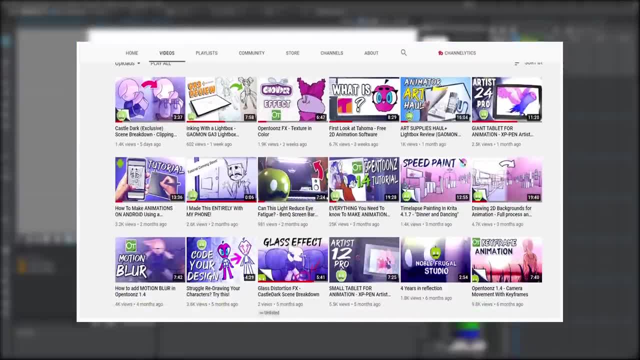 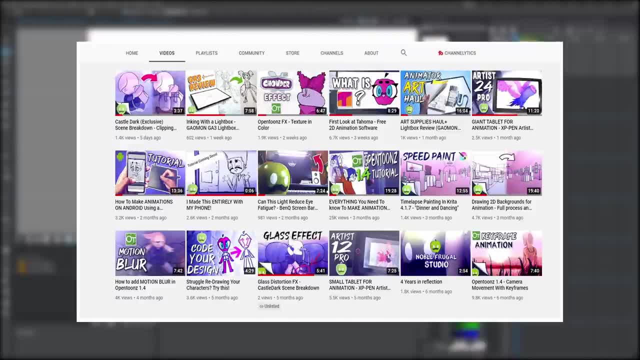 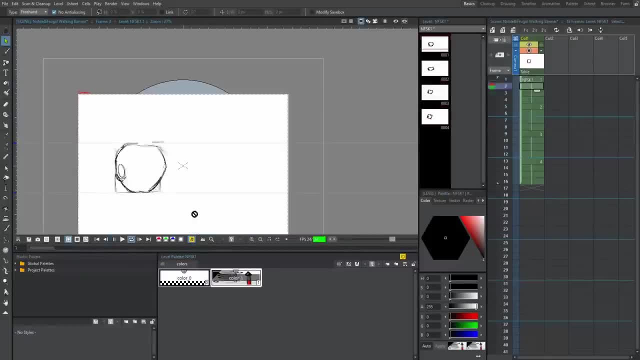 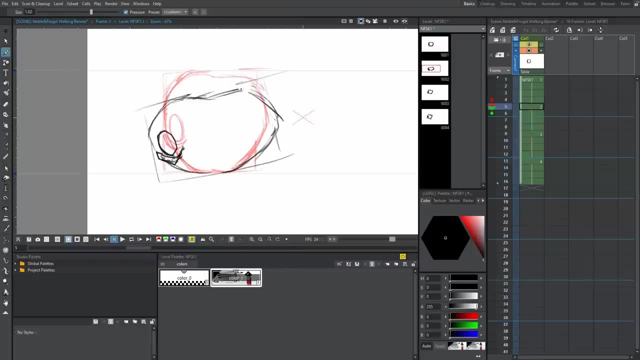 A YouTube channel can also act as the home base for your Internet brand. Otherwise, if you're new to animation, you might want hold off sharing until you've considered a few things. What I see online all the time, especially with really young people, is that they'll 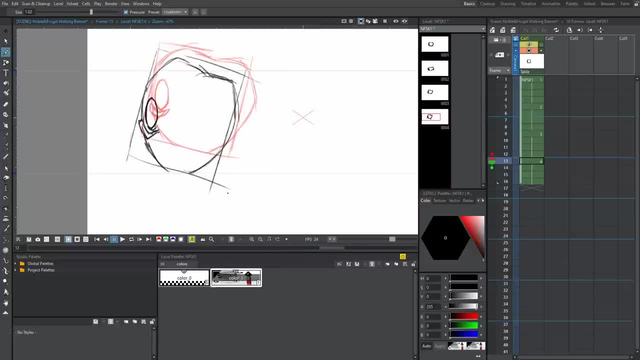 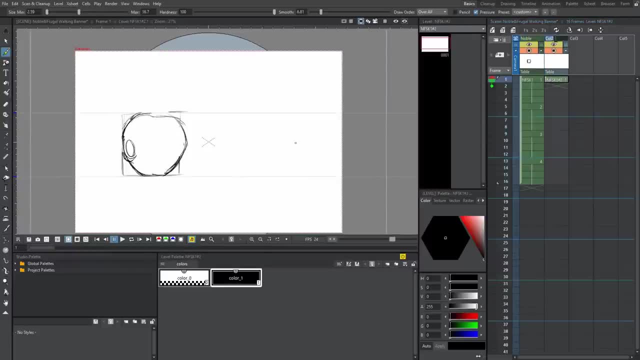 share their rudimentary or really low effort work online and then just get blasted by others for it. This is just really painful to see and can be hurtful to the artist and the community as a whole. This happens so often that I frequently see people share an animation. 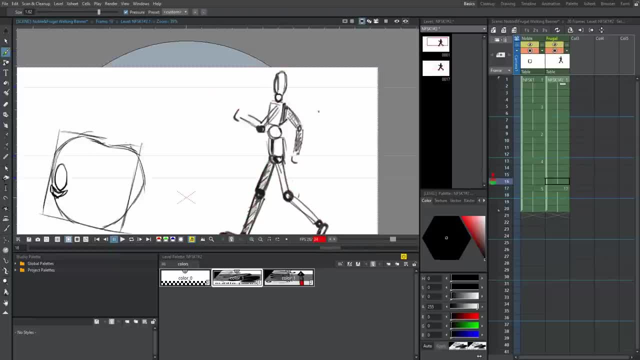 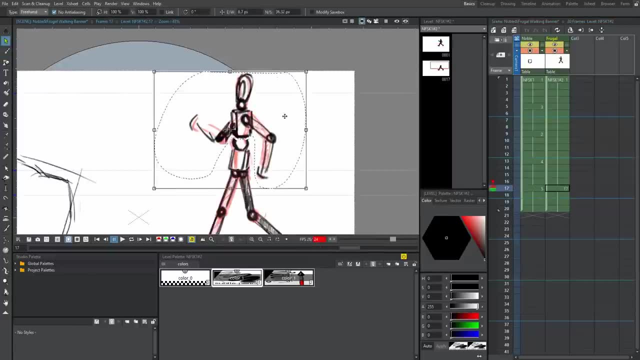 and they'll say it's not good, or I know it's bad, but here it is anyway, etc. And I believe they say these things so that people don't blast them, but what they're really doing is ruining their self-esteem and their confidence in their own work. 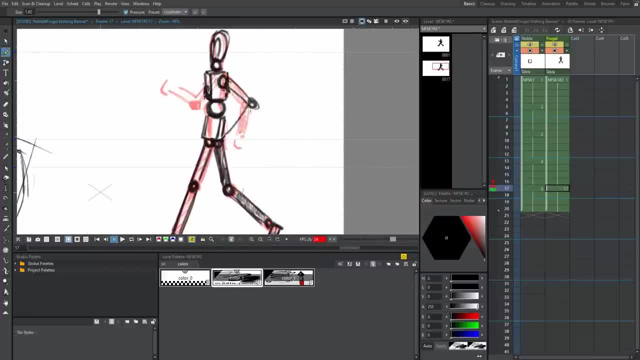 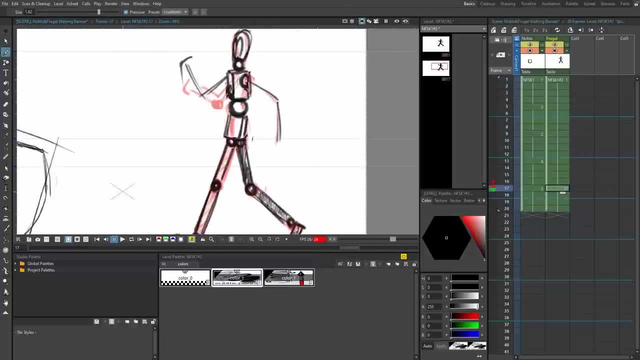 It takes a lot of work to master any skill, so why should drawing an animation be any different? If your first few animations don't look good, it just means that you have a lot of practice to do. You can't really be bad at something that you don't have experience in. 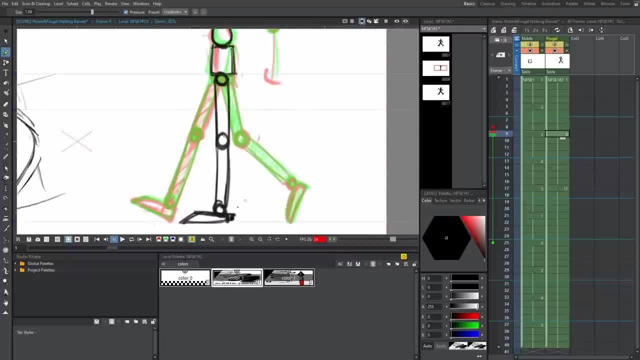 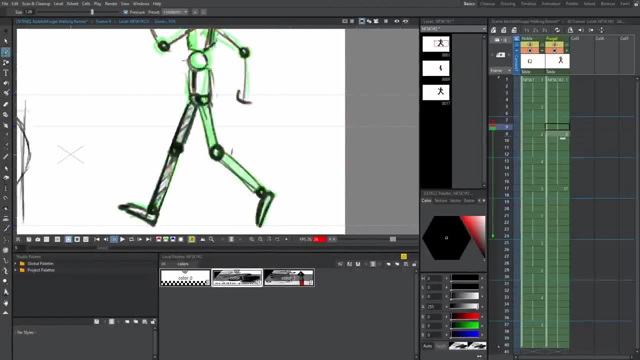 But also, if you're going to share your work online with a bunch of unknown people, make sure you know what you're getting into. Once you start animation, how do you get better? There are 12 main principles of animation that teach you the basics. 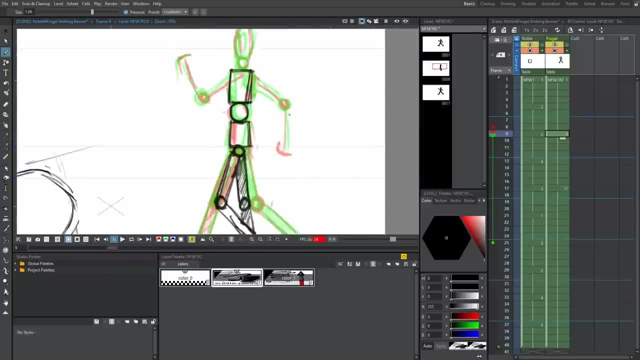 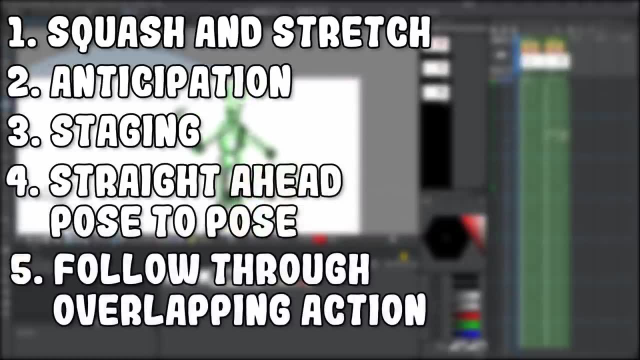 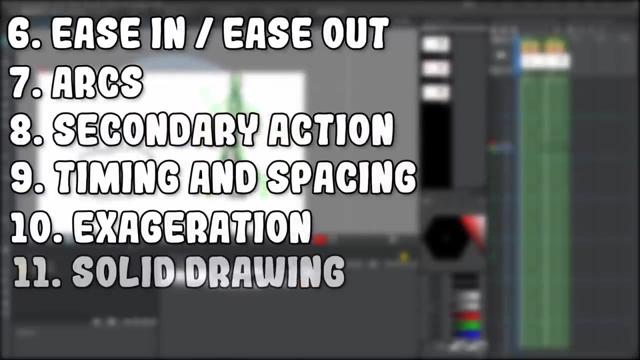 If you get to know these well, your animations will start looking professional. The 12 principles are: squash and stretch, anticipation, staging straight ahead and pose to pose, follow through in overlapping action, ease in and ease out arcs, secondary action, timing, exaggeration, solid drawing and appeal. 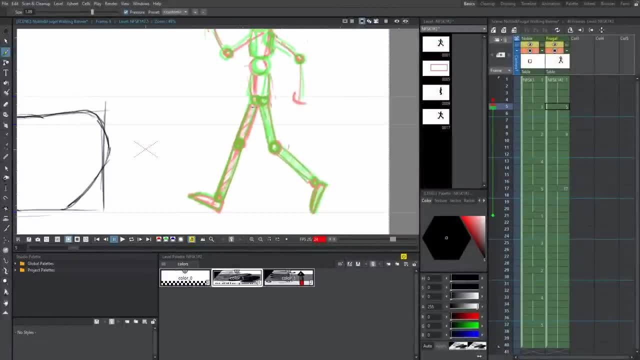 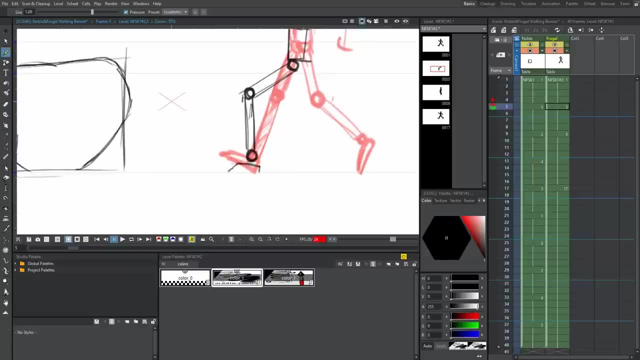 Once you master these basic principles, you can go on to the more advanced ones, which demonstrate different types of motion. These include the wave principle, counterposing, breaking joints, accents, leading action, etc. There's a lot. All of these are summarized in this neat video called. 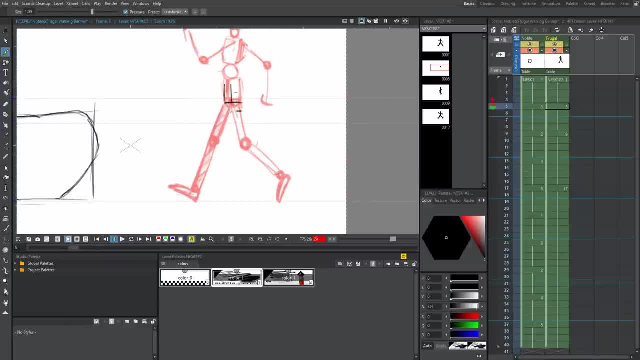 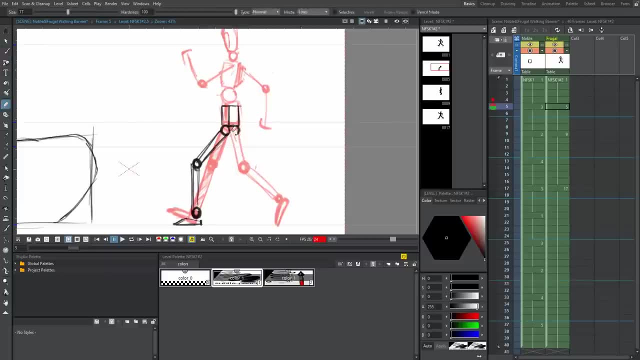 The 21 Foundations of Animation by The Angry Animator. Once you master each one of these principles, you'll be a highly skilled animator, ready for any project. At that point, you can go on to study motion by observing life around you, keenly to discover how you can capture it more effectively. 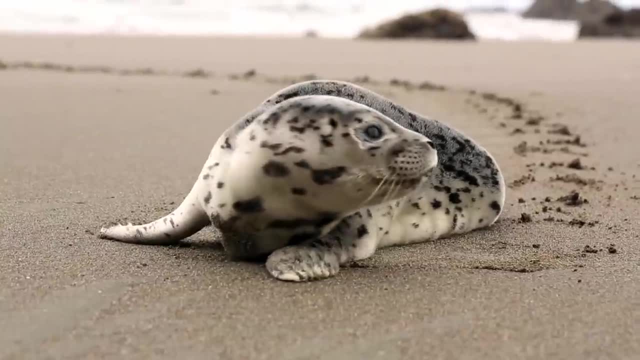 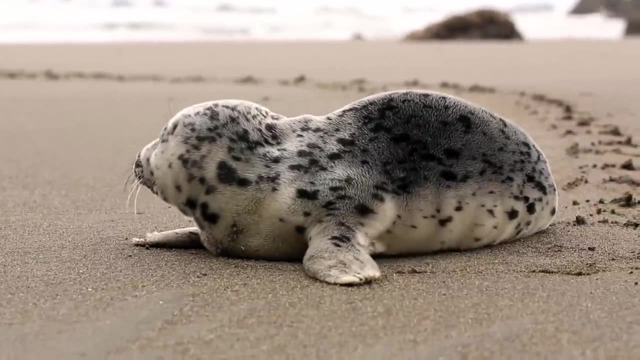 After thorough study, you'll probably develop your own principles of animation. The point is that you'll never truly master animation, just as no one can ever be the one true master at any skill. We can definitely get really good at it, but the world around us is far too complex, intricate and beautiful to ever truly replicate it. 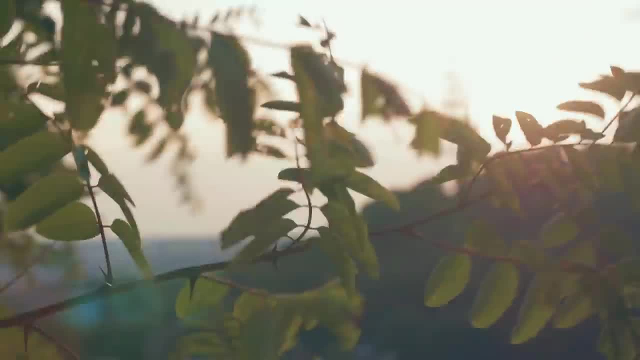 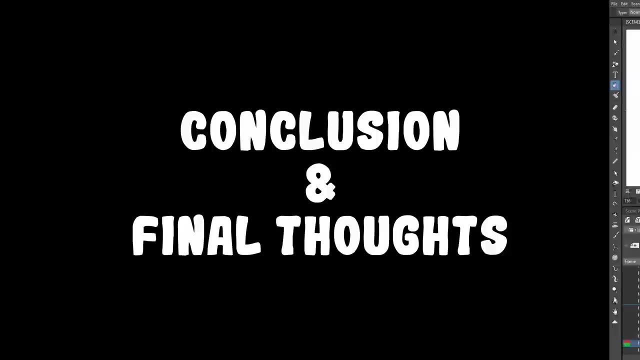 The good thing, though, is that we don't have to replicate real life. In fact, you can just focus on what appeals to you and bring that out in your work. Conclusion and final thoughts: Animation is a complicated art, so don't beat yourself up if you can't get past. 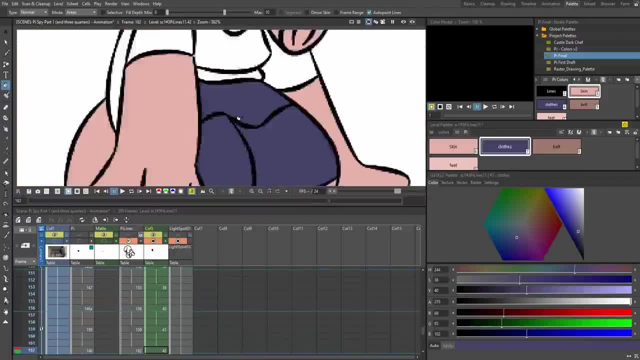 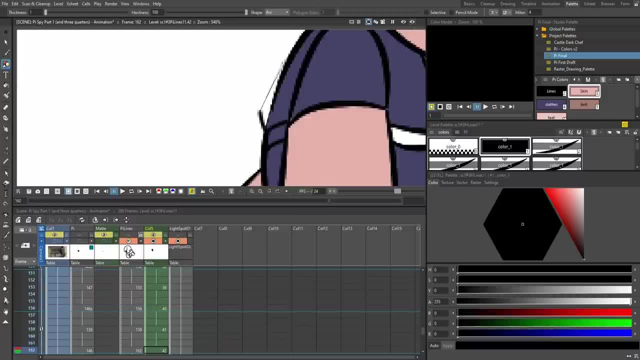 a certain exercise or your animation isn't looking how you want it to. That's easier said than done. You know the not beating yourself up part, But as long as you focus on mastering the basics first, your journey should stay on track. 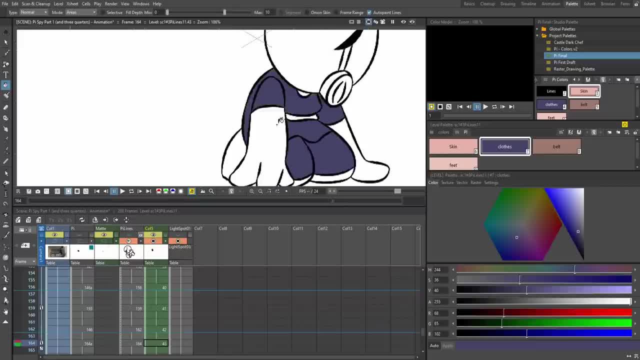 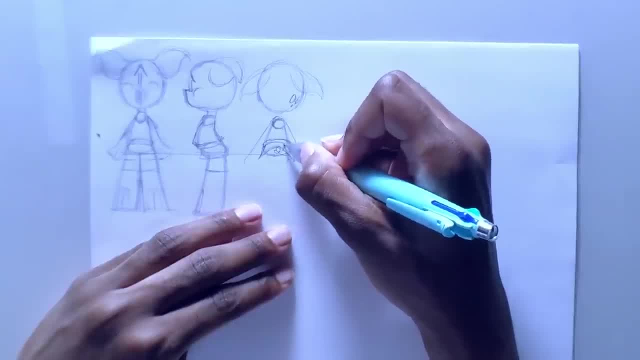 One thing I'd like to mention is that making 2D animations requires drawing skills, And now, before you click away, I want to say: don't be afraid to learn how to draw. Drawing is a really underrated life skill that can help you in a multitude 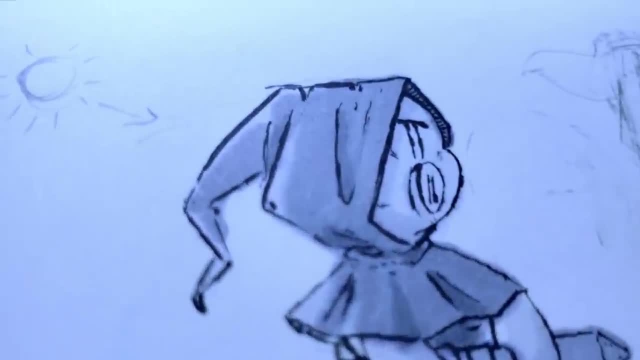 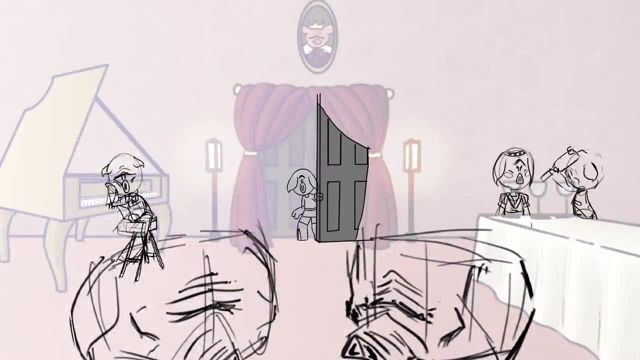 of arenas. Learning how will take time, but that's not reason to toss it out the window. All skills take time. In order to gain proficiency in any skill, you have to practice, you have to fail, you have to succeed, But most of all, you have to learn.